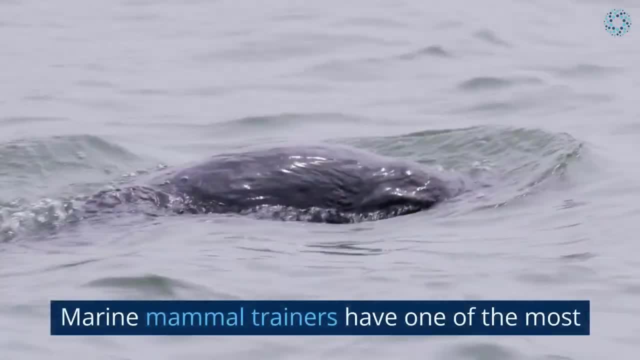 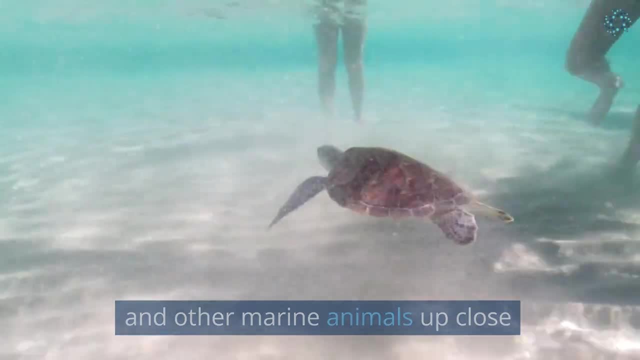 Number 10. Marine Mammal Trainers. Marine mammal trainers have one of the most exhilarating jobs out there. They bring dolphins, sea lions and other marine animals up close and personal with visitors at marine parks and aquariums. According to, Comparably, the pay for marine 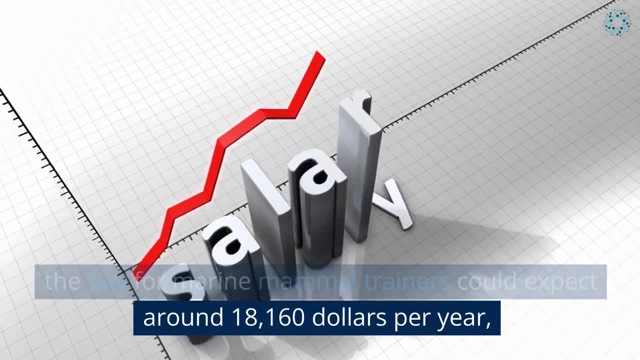 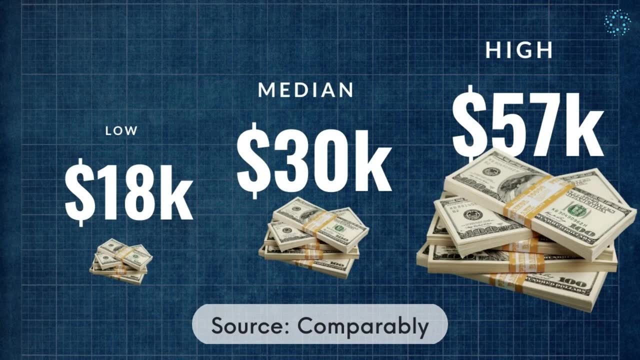 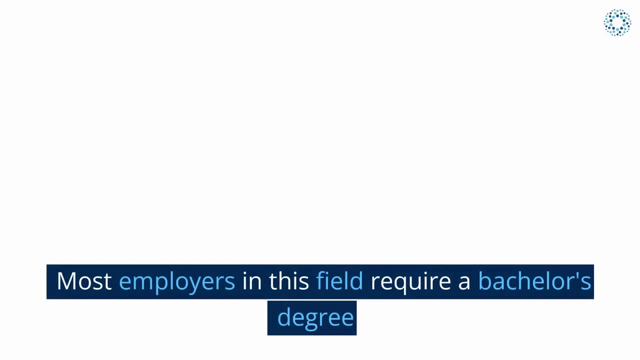 mammal trainers could expect around $18,100 per year, While on the higher end it can reach up to an impressive $57,170 per year. The median pay falls around $30,328 annually. Most employers in this field require a bachelor's. 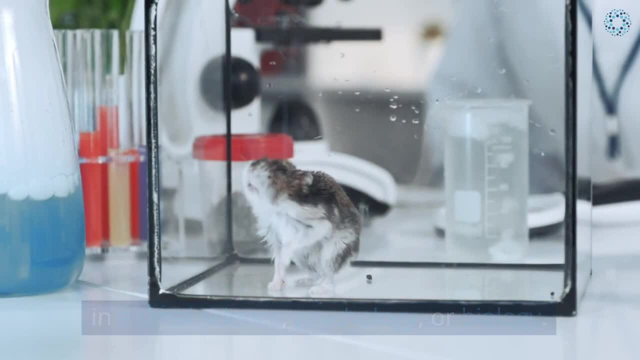 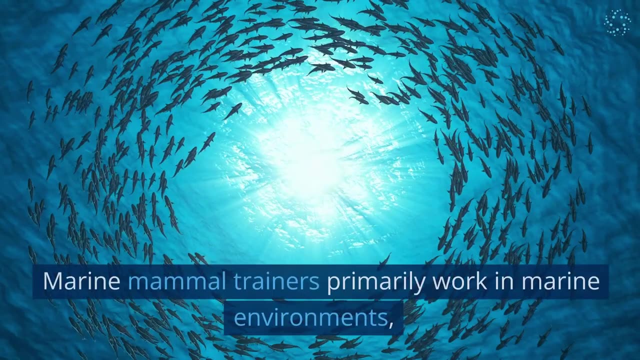 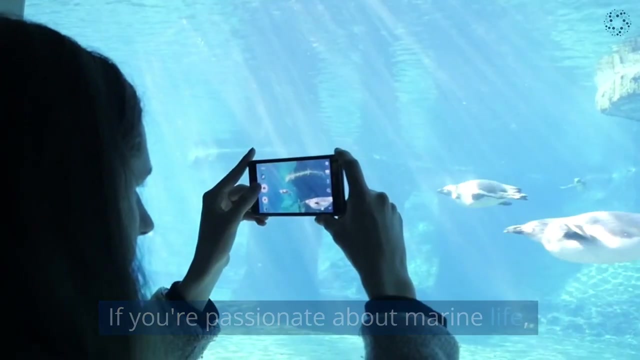 degree in animal science, psychology or biology. Strong communication skills are also vital, as you'll be interacting directly with customers and visitors. Marine mammal trainers primarily work in marine environments such as aquariums and marine parks. If you're passionate about marine life. 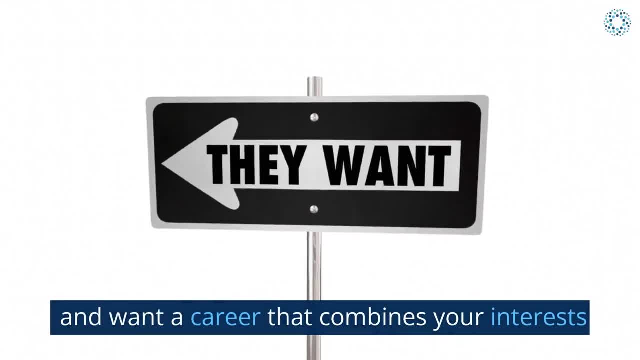 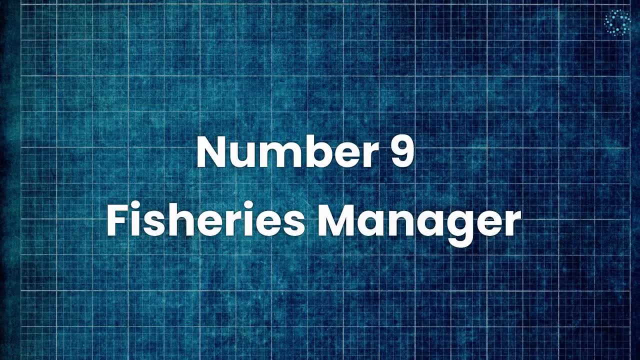 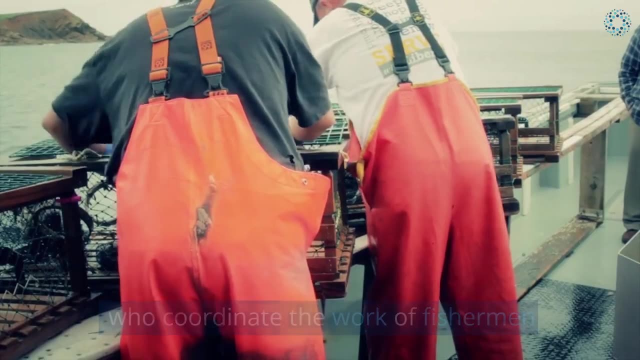 love working with animals and want a career that combines your interests with an exciting and rewarding environment, becoming a marine mammal trainer could be your perfect fit. Number 9. Fisheries Manager. Fisheries managers are dedicated professionals who coordinate the work of fishermen and 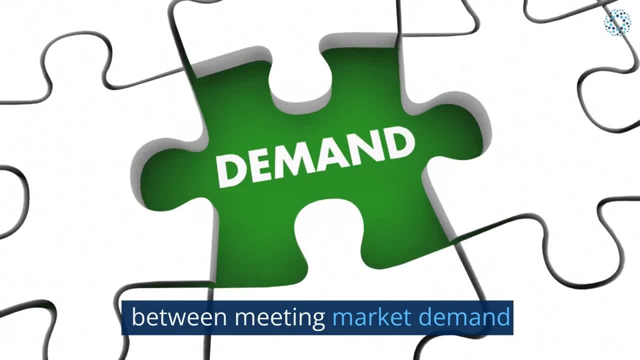 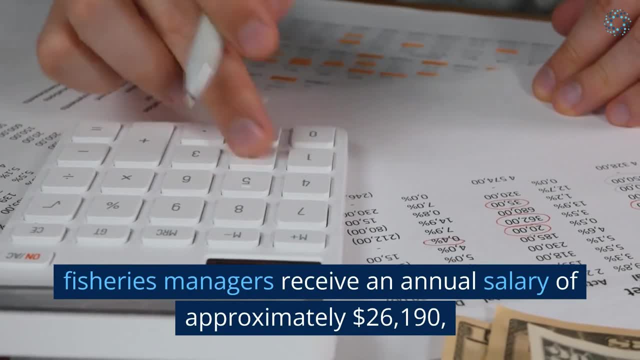 fisherwomen. striking a delicate balance between meeting market demand and protecting our marine ecosystems Comparably reveals that fisheries managers have the ability to cater to all of our Receivers, receive an annual salary of approximately $26,190,, with the high rent reaching a remarkable 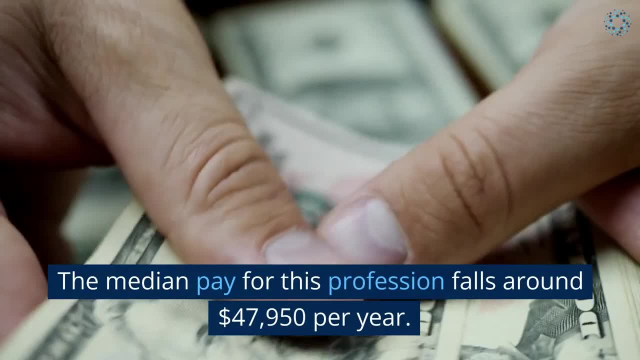 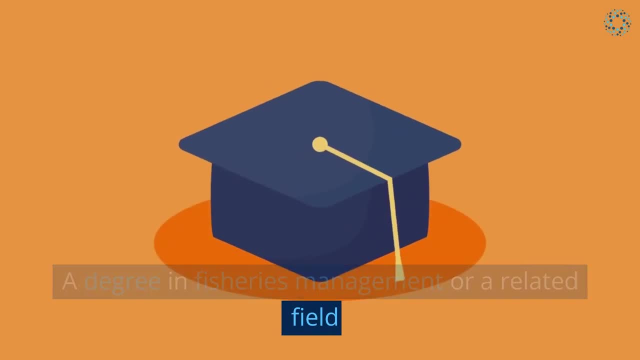 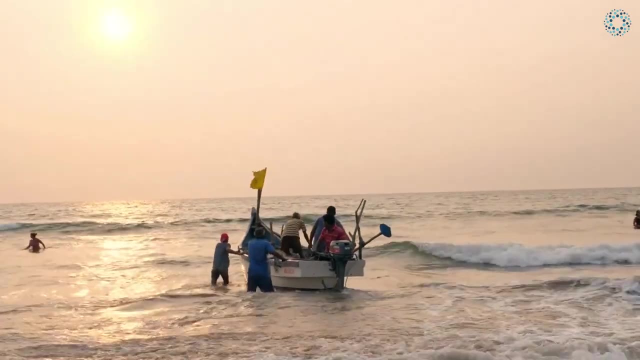 $97,390.. The median pay for this profession falls around $47,950 per year. A degree in fisheries management or a related field is typically required, and possessing management and leadership skills is vital to excel in this position. If you're ready to dive into the rewarding world of fisheries management, explore the. 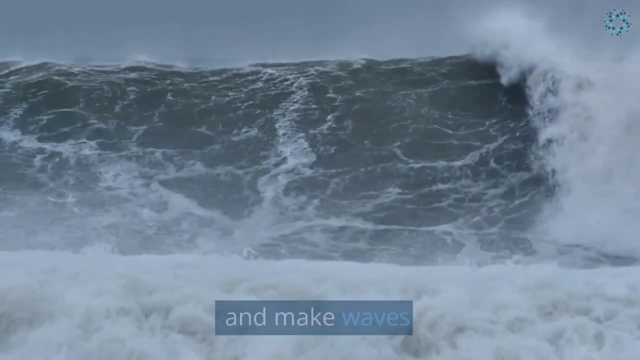 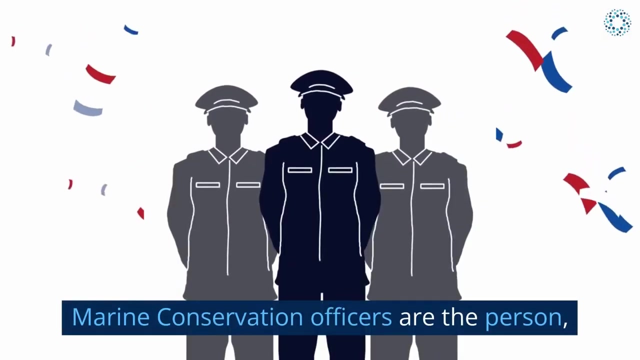 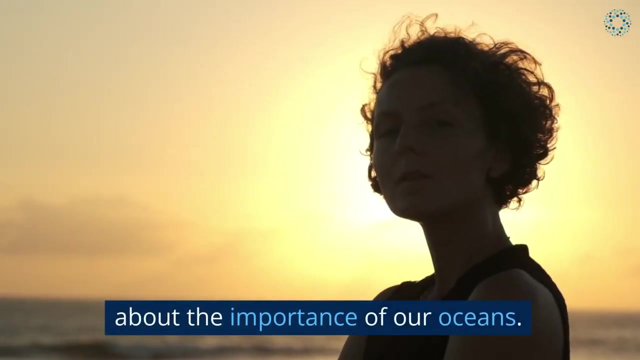 possibilities, gain the necessary skills and make waves in conserving our precious marine resources. Number 8. Marine Conservation Officer. Marine Conservation Officers are the person who safeguard marine life, enforce conservation laws and educate the public about the importance of our oceans. 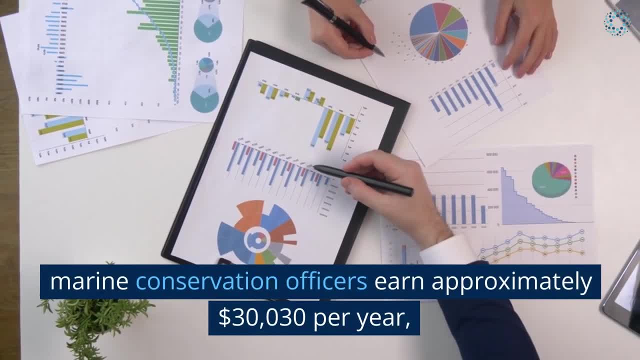 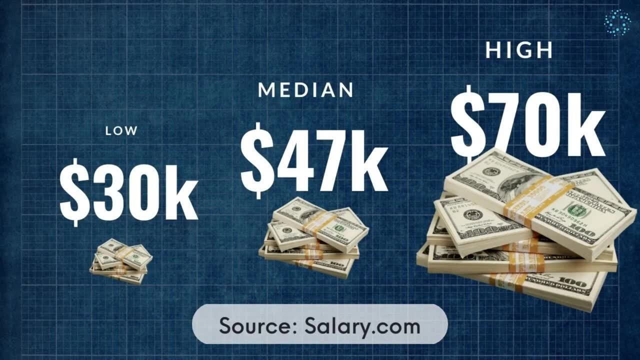 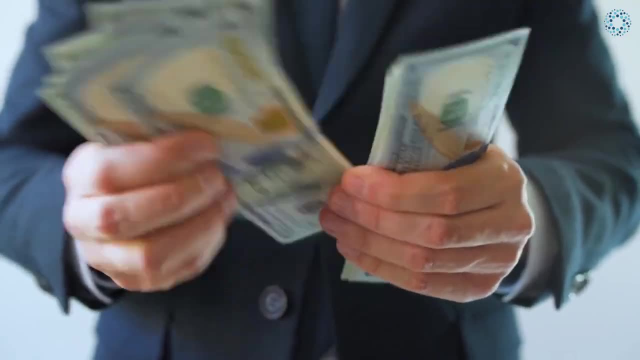 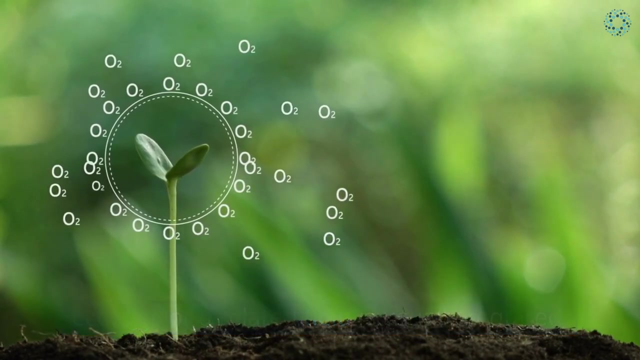 Salarycom reports that Marine Conservation Officers earn approximately $30,030 per year, with the high rent of the pay scale reaching an impressive $70,613.. The median pay for this profession falls around $47,998 per year. A bachelor's or master's degree in biology, ecology or a related field is usually required. 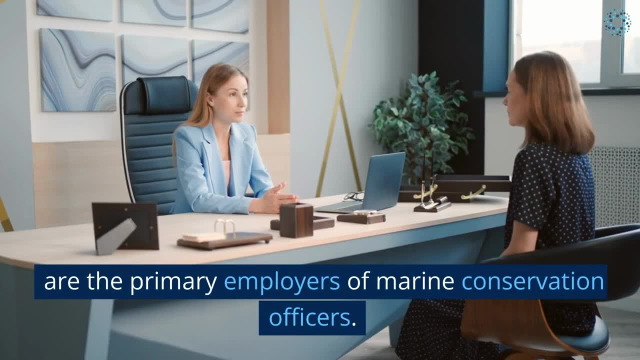 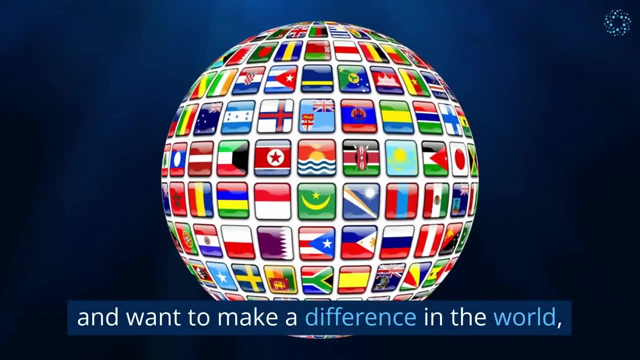 Government agencies and non-profit organizations are the primary employers of Marine Conservation Officers. If you're passionate about marine life, have a deep love for the ocean and want to make a difference in the world, becoming a Marine Conservation Officer could be your perfect fit. 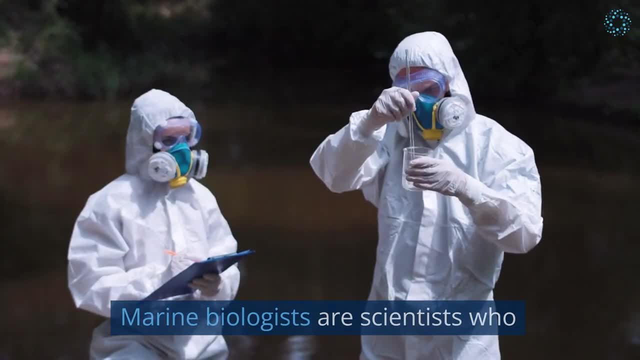 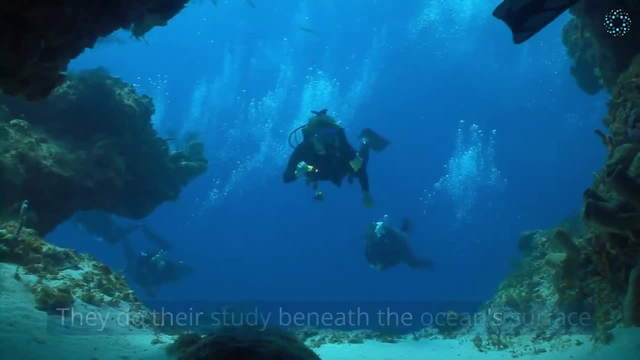 Number 7. Marine Biologist. Marine Biologists are scientists who dive into the depths to study marine life and unravel its secrets. They do their study beneath the ocean's surface, where a world full of awe-inspiring creatures and mesmerizing ecosystems lies. 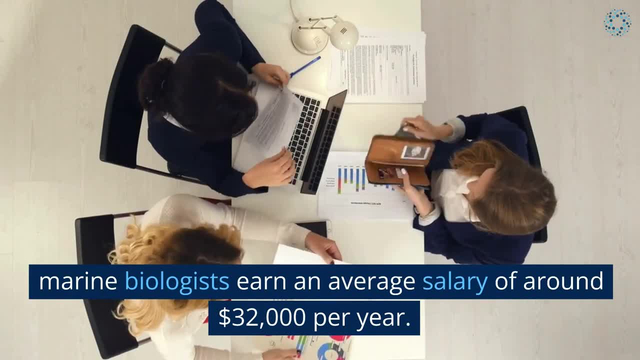 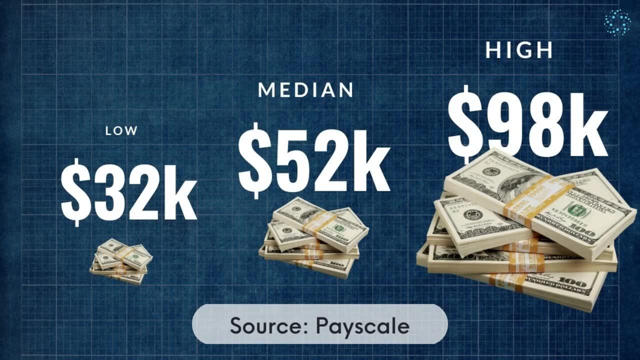 Based on pay scale data, Marine Biologists earn an average salary of around $32,000 per year. However, at the higher end, their pay can reach an impressive $98,000 annually. The median pay for this profession stands at $7,000. 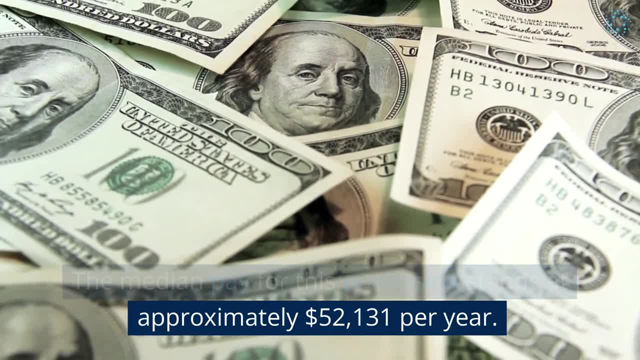 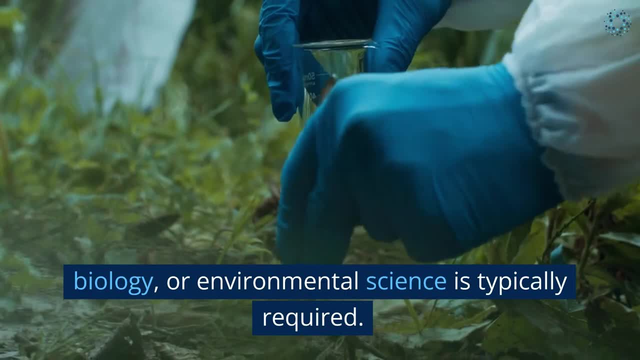 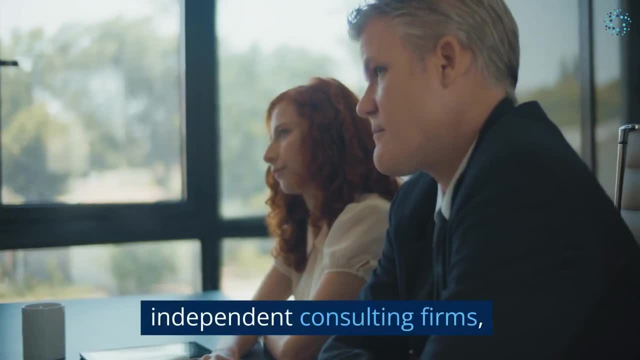 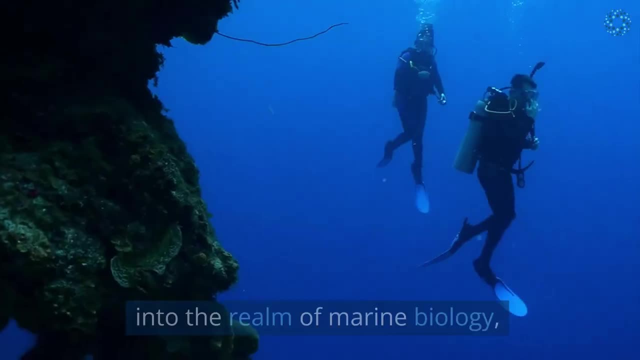 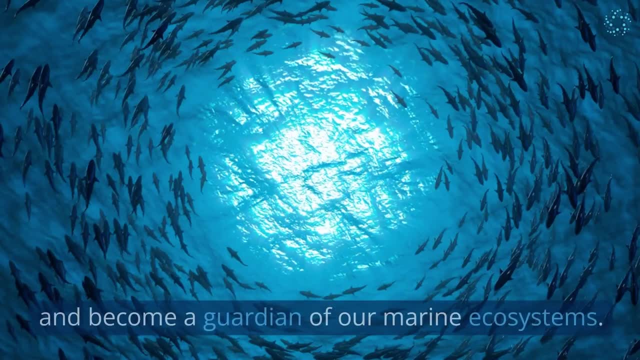 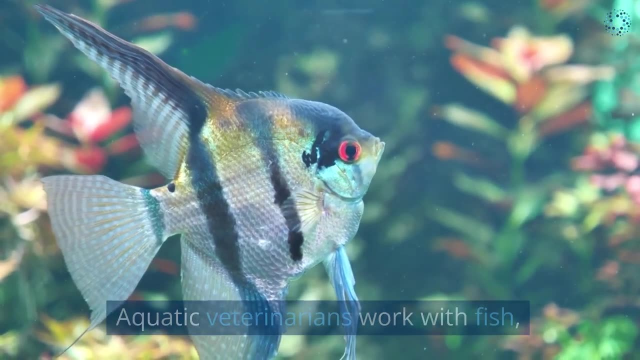 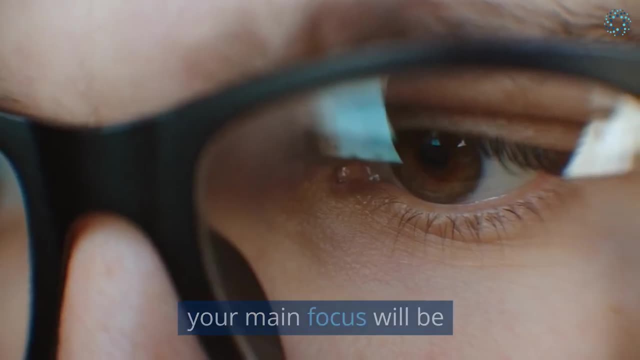 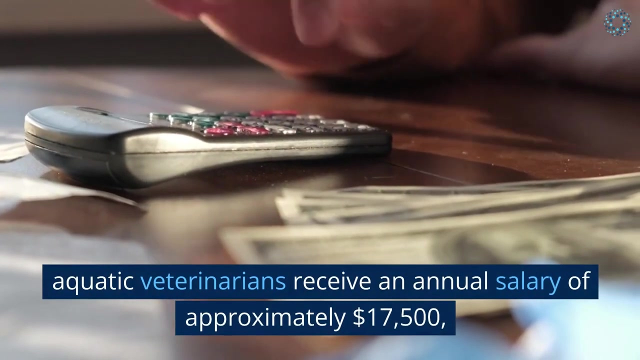 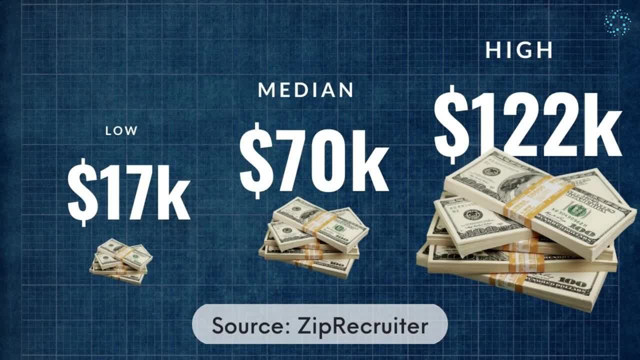 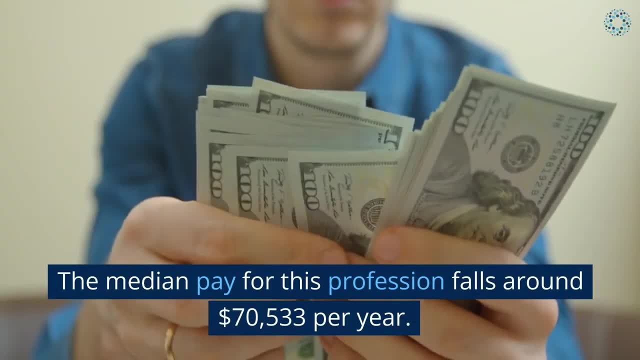 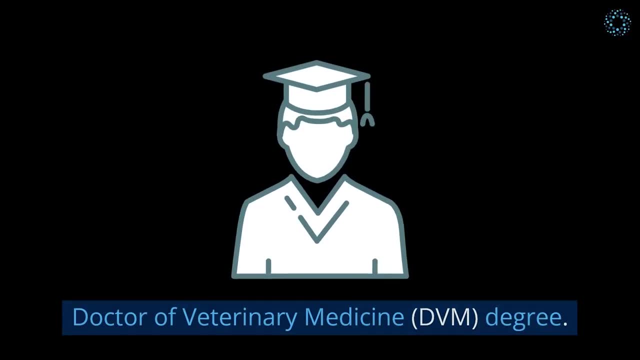 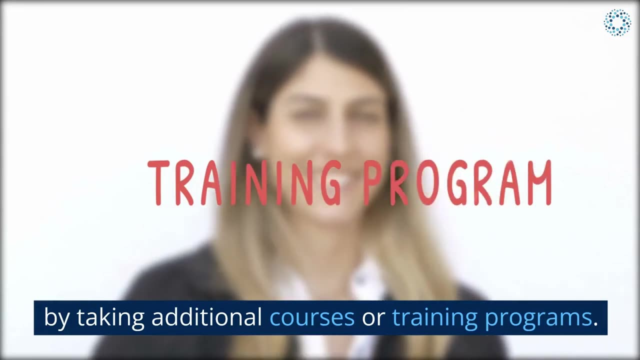 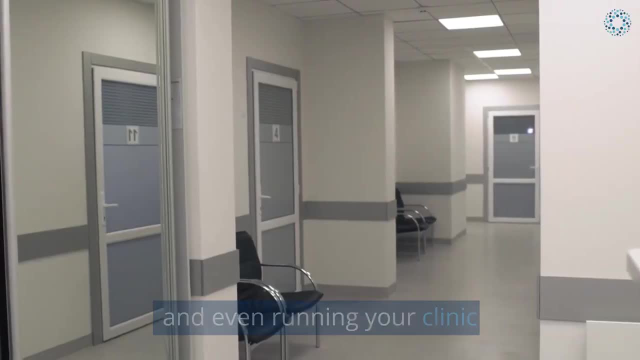 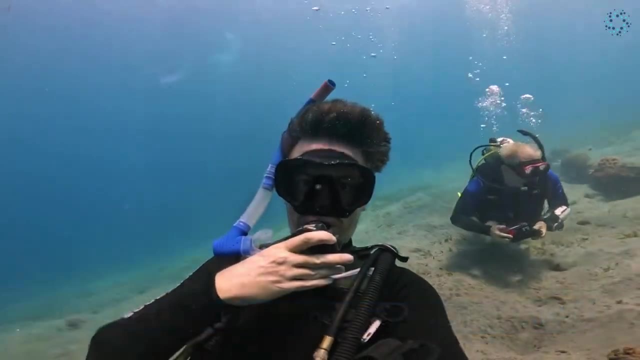 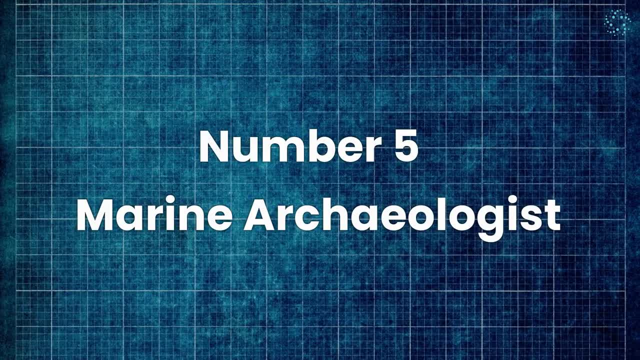 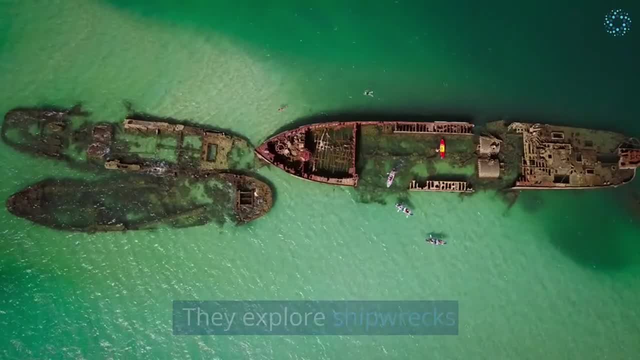 the health and welfare of aquatic life. Number 5. Marine Archaeologist. Marine archaeologists study the history and mysteries hidden beneath the waves. They explore shipwrecks and uncover the secrets of the past. As a marine archaeologist, your work will revolve around underwater. 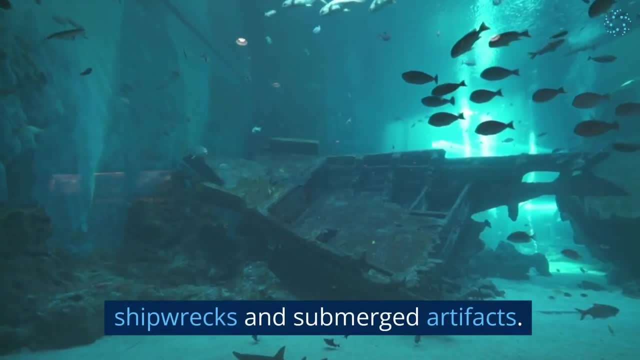 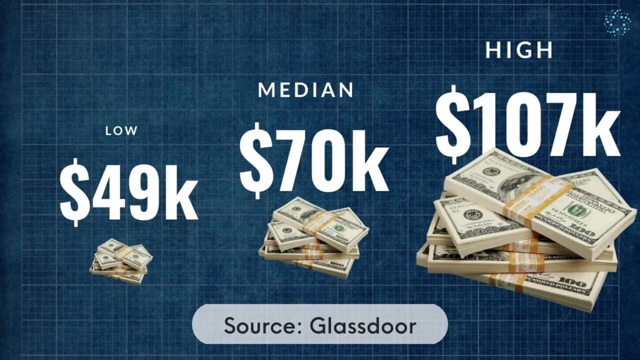 archaeology, which involves investigating shipwrecks and submerged artifacts. Glassdoor Dot reveals that marine archaeologists receive a competitive salary. The salary range for this profession can vary, starting at approximately $49,000 per year and reaching as high as $107,000. 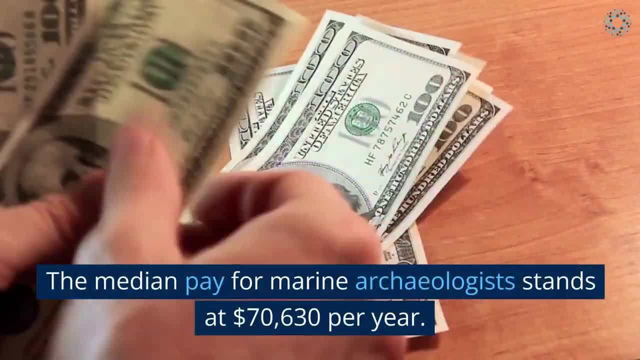 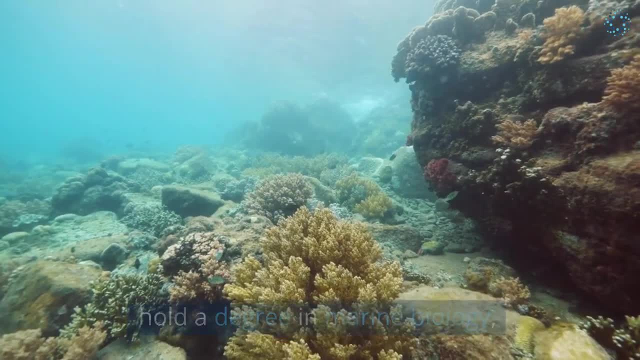 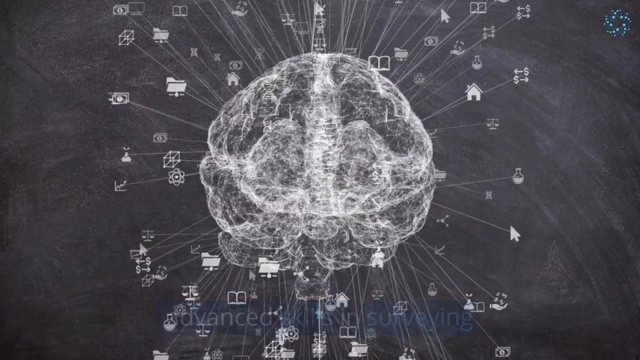 per year. The median pay for marine archaeologists stands at $70,630 per year. To enter this field, many professionals hold a degree in marine biology, anthropology or archaeology. However, for specialized roles that require advanced skills in surveying, 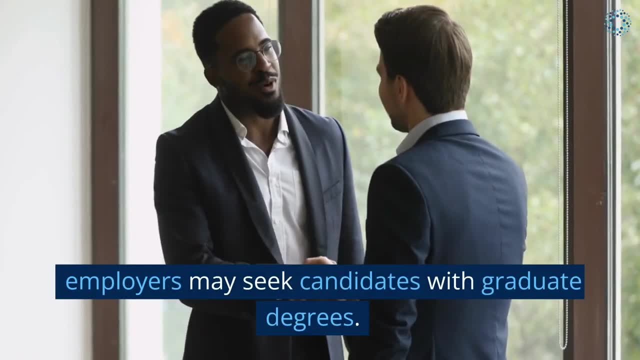 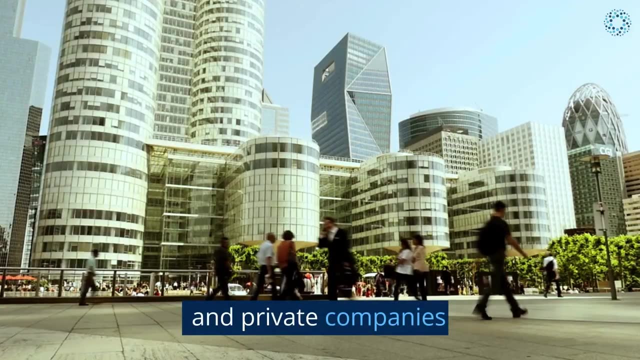 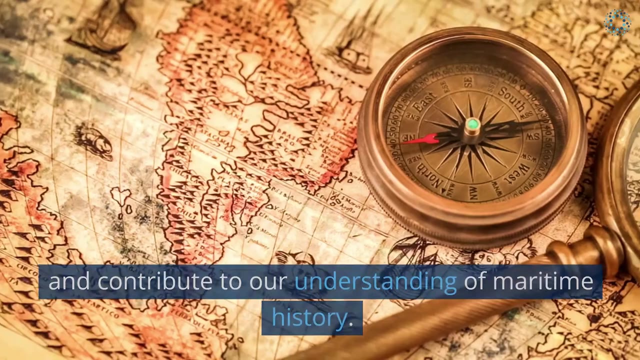 and underwater excavation techniques. employers may seek candidates with graduate degrees. Museums, universities, government agencies, corporations and private companies all seek the expertise of marine archaeologists. You'll have the chance to work on fascinating projects and contribute to our understanding of maritime history If you're ready to dive into a career. 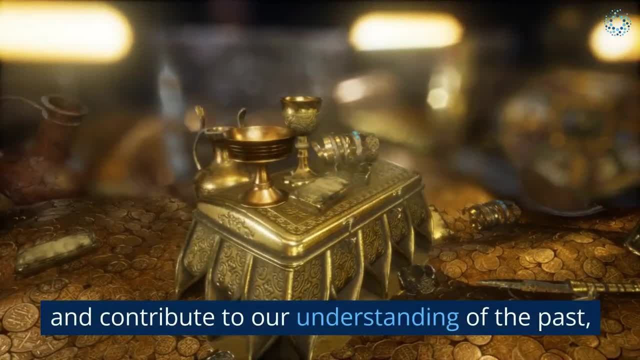 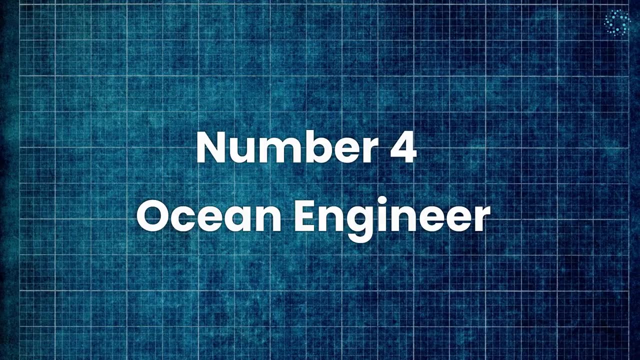 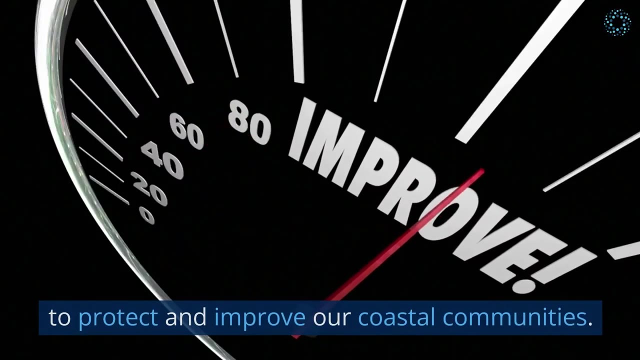 that allows you to uncover hidden treasures and contribute to our understanding of the past. pursue your education and become part of the Marine Archaeologist. 4. Ocean Engineer. Ocean Engineers are the unsung heroes working behind the scenes to protect and improve our coastal communities. As an ocean engineer, your primary role is to manage and maintain systems that ensure the cleanliness and safety of our oceans. According to Salarycom, the median annual salary for ocean engineers ranges from $47,571 to $102,077.. The median pay stands at a respectable $72,009 per year. To enter this field, a bachelor's degree in engineering. 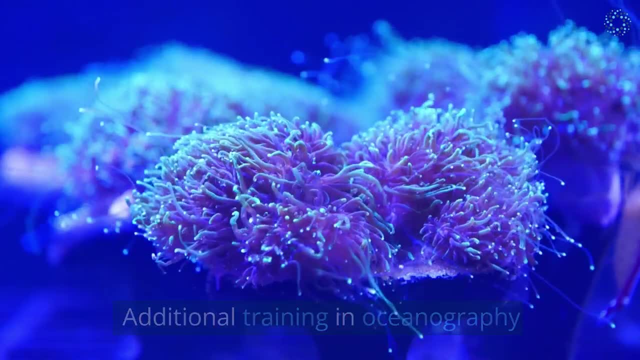 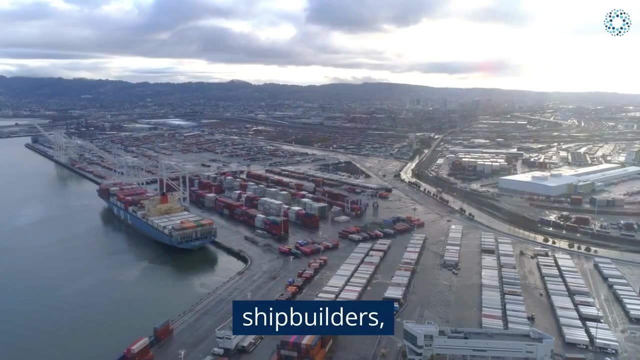 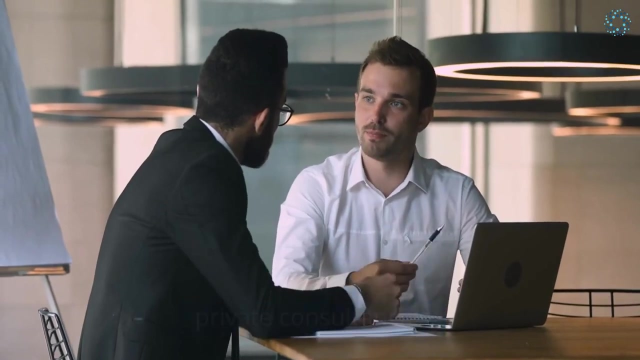 or science is typically required. Additional training in oceanography or marine biology can also be beneficial. Potential employers for marine engineers include shipyards, shipbuilders, port authorities, tidal power plants, research labs, government agencies, private consultancies and water transport industries. If you're ready to build the future of our oceans, start by. 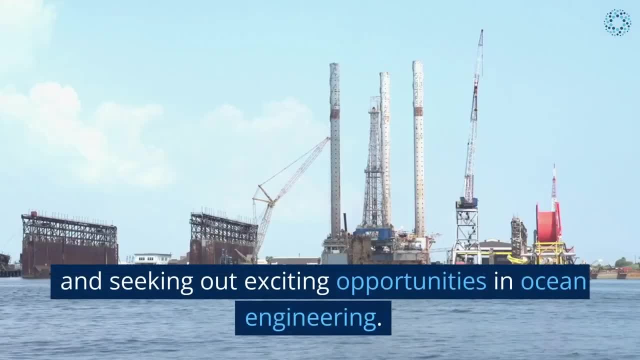 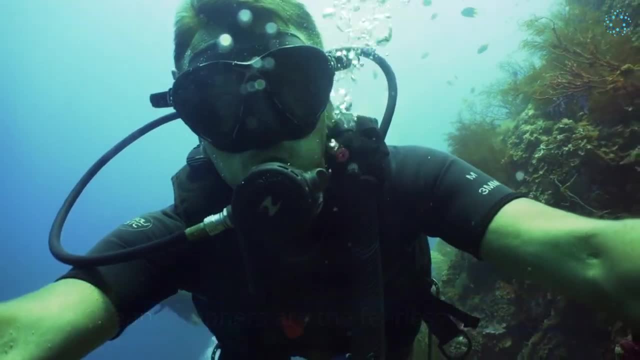 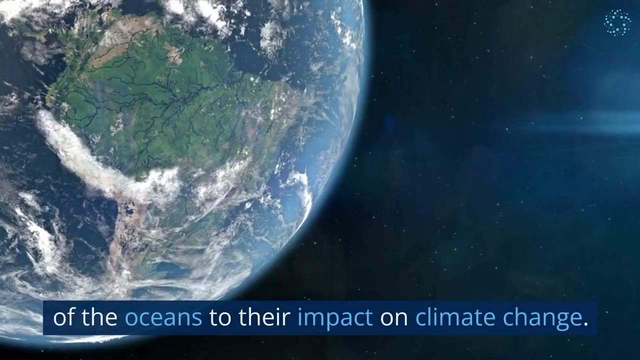 acquiring the necessary education and seeking out exciting opportunities in ocean engineering. 3. Oceanographer: Oceanographers are the fearless explorers who unveil the mysteries of our deep blue planet. As an oceanographer, you'll study everything from the chemistry of the oceans to their impact on climate change. Salarycom reports. 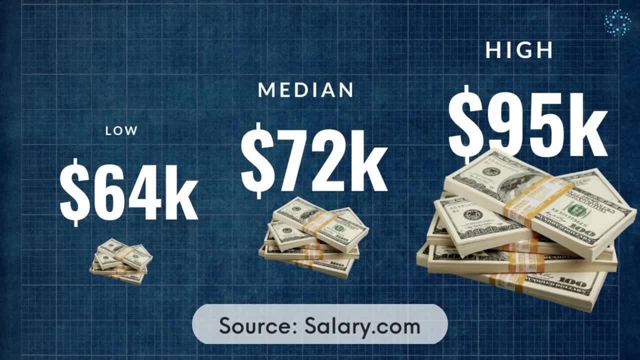 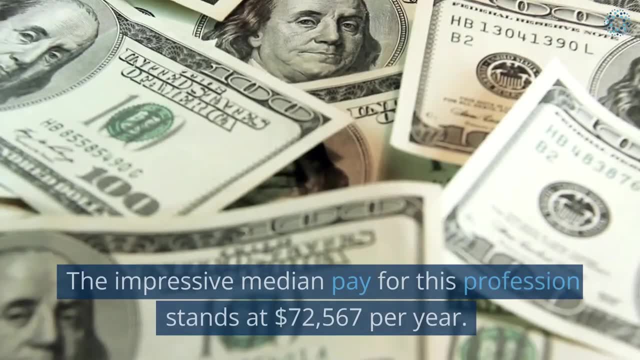 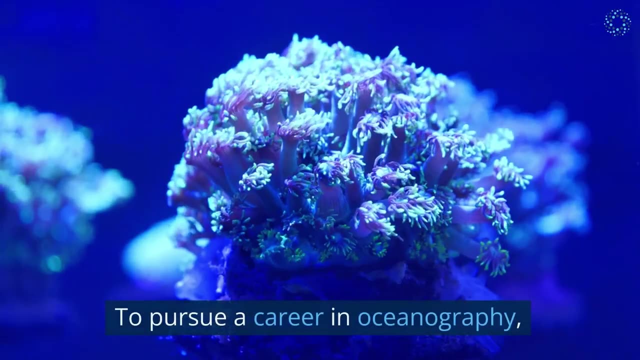 that oceanographers can expect a median annual salary ranging from $64,253 to $95,900 per year. The impressive median pay for this profession stands at $72,567 per year. To pursue a career in oceanography a bachelor's degree in oceanography or a related field. 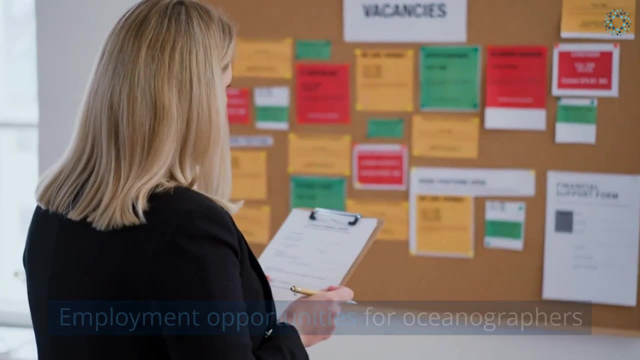 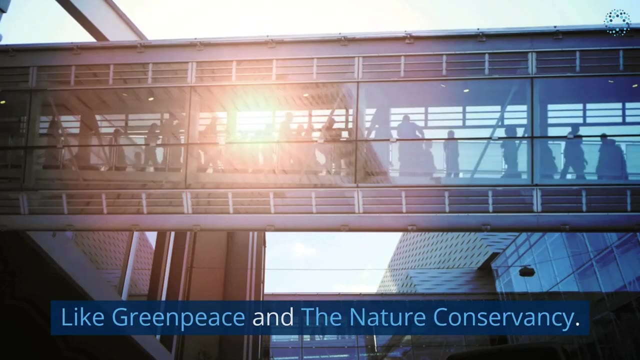 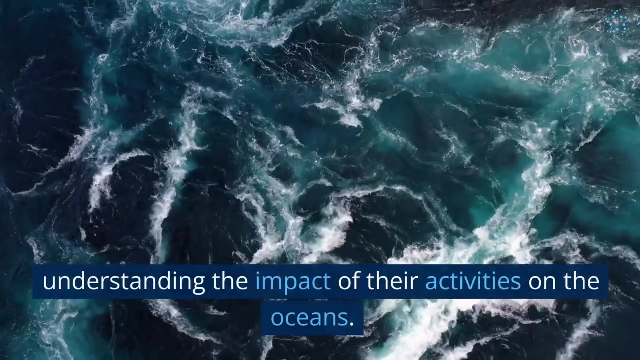 is typically required. Employment opportunities for oceanographers can be found at universities, research centers and environmental organizations like Greenpeace and the Nature Conservancy. Moreover, oceanographers are sought after by oil companies and other businesses, and many of them are interested in understanding the impact of their activities on the oceans. 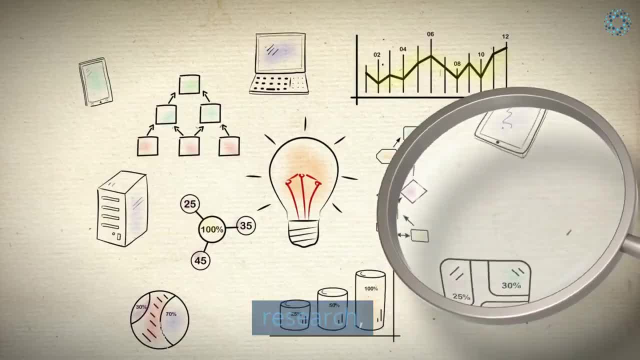 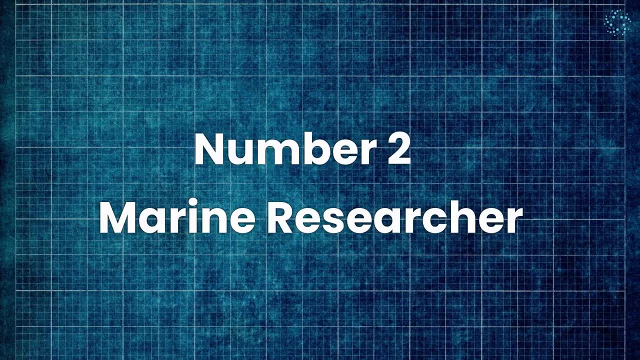 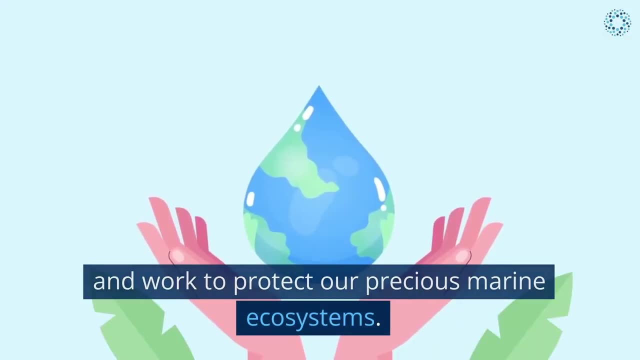 If you're ready to dive into a career filled with discovery, research and exploration, begin your journey by pursuing a degree in oceanography or a related field. 2. Marine Researcher. Marine researchers are scientists who unlock the mysteries of the deep and work to protect our precious marine ecosystems. As a marine 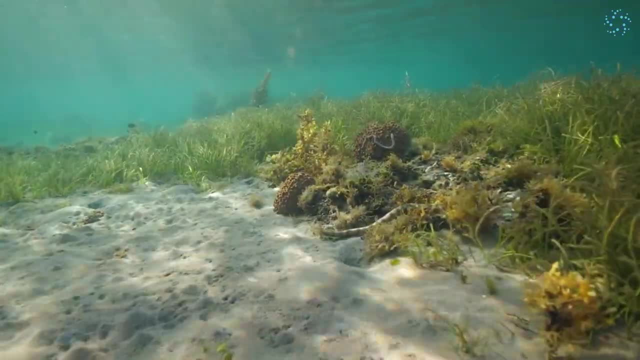 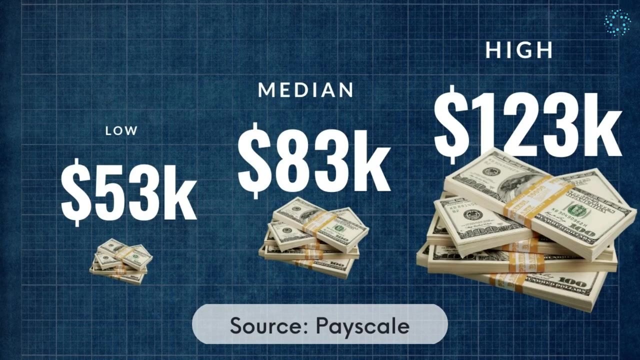 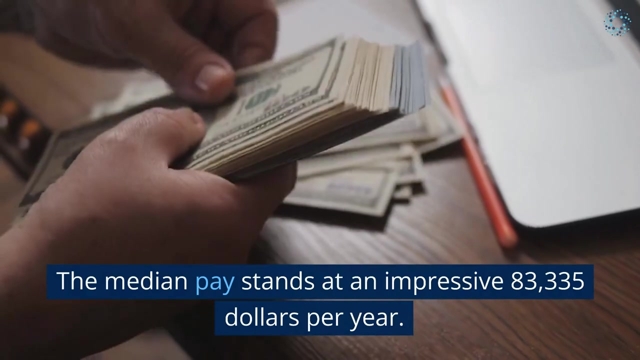 researcher, your primary focus will be studying ocean life and assessing the impact of human behavior on marine life. As a marine researcher, you'll study the impact of human behavior on marine ecosystems. According to Payscale, marine researchers earn a median annual salary ranging from $53,000 to $123,000. The median pay stands at an impressive $83,335 per year.